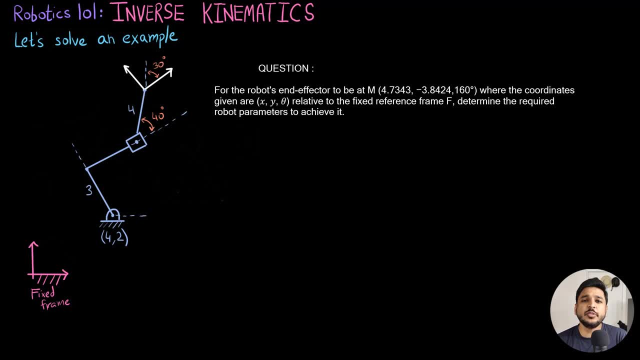 Hi and welcome back to Robotics 101.. In this video we are going to do a very interesting problem of inverse kinematics. So I have a robot here which is displaced from the fixed frame: four units in x and two units in y. It has a link right here which has a dimension of three units and 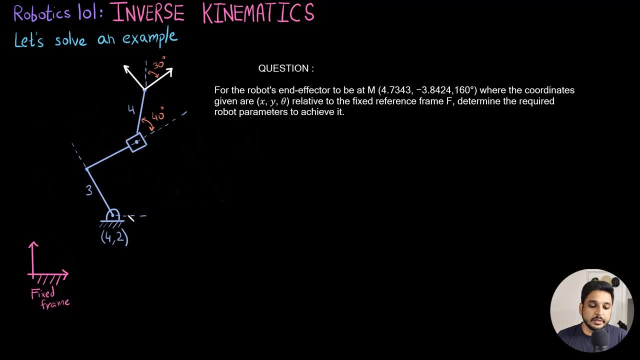 there's a motor attached right here, So this link can rotate and the rotation angle is represented by theta one. Now this is my second link. Again, this link can rotate too, and the rotation angle is marked by theta two. here And this right here is a prismatic joint. So it means that this joint 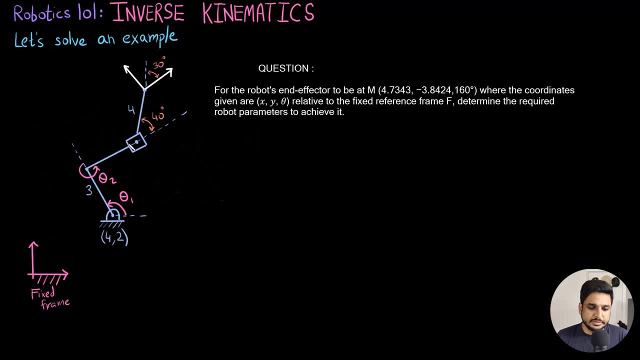 can extend or retract, So this length is variable. So I just call this the length of this link as L2.. Now I have another link here which is fixed. It is fixed at an angle of 40 degrees and has a dimension of four units and the end effectors. 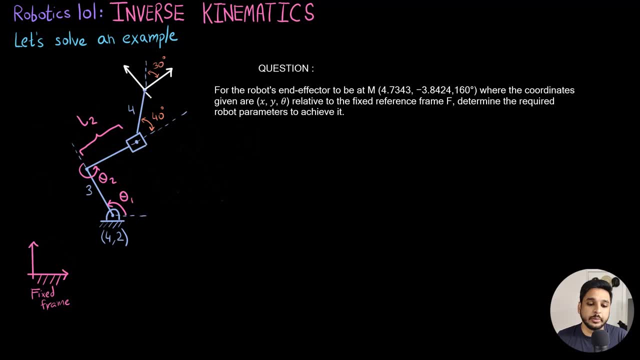 again fixed at a treated angle of 30 degrees. So this is my end effectors frame right here. So now coming to the question. So the question is for the robot's end effector to be at m, which has this x, this y and this orientation, where the coordinates given are x, y and theta relative to 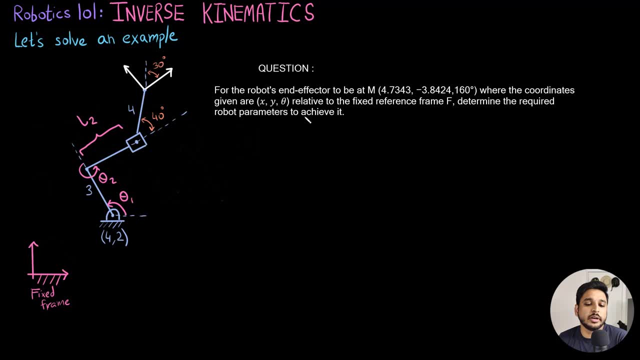 the fixed reference frame Determine the required robot parameters to achieve it. So this is what my end effector's moving frame should be. So, in short, my end effector's frame should be at the required position. So this represents my x coordinate of the end effectors. 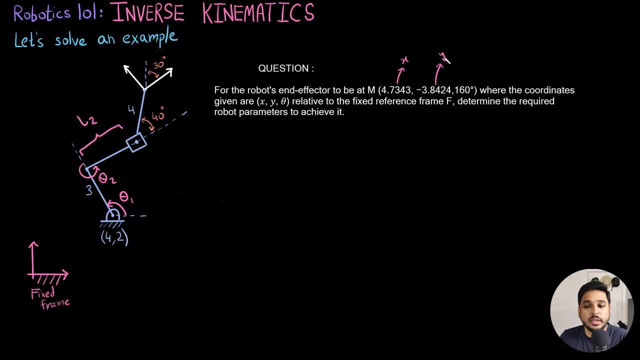 This coordinate represents my y coordinate of the end effectors frame and this angle, 160 degrees, represents the orientation of the end effector. Let me mark it as theta. So what I can do is I can write this in this form. So I am given this and I know that this. 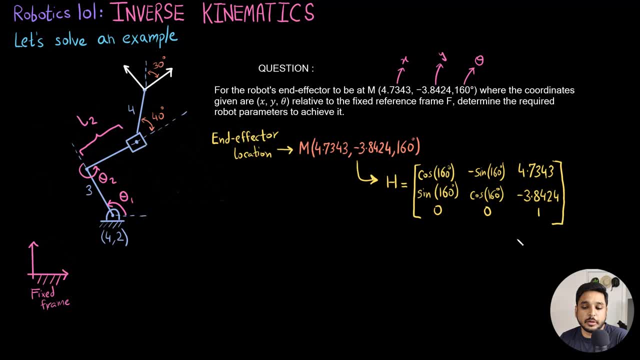 can be written in a homogeneous form in this manner, which just has a rotation matrix here, with the angle as 160 degrees, and this is my x and this is my y. Now, the way to do this problem is, since it is an inverse kinematics problem, so what you do is you. 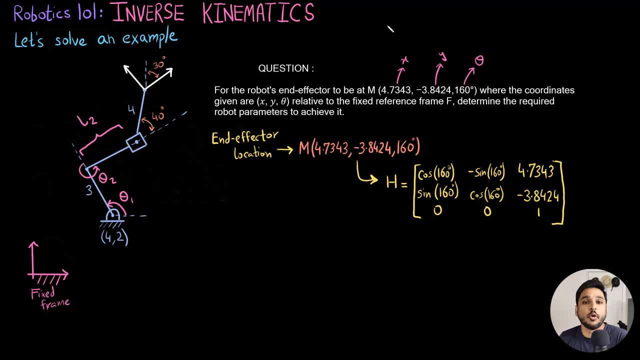 first do the forward kinematics software. So the way you can do this is simply by First considering all the homogeneous transforms. that takesINDEX to the forward kinematics. Let's see how this works. the robot's end effector from the fixed frame. so it takes the fixed frame to the robot's end. 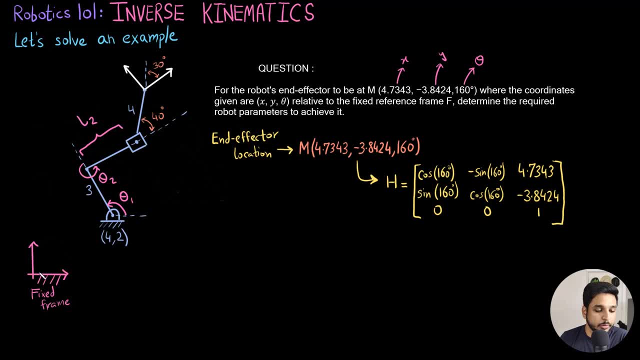 effector frame. so, going from here to here, i can say that there is a homogeneous transform which takes the fixed frame to this point. i call it h0. then there is another homogeneous transform that just rotates the frame here. so i call this homogeneous transform h1, which has 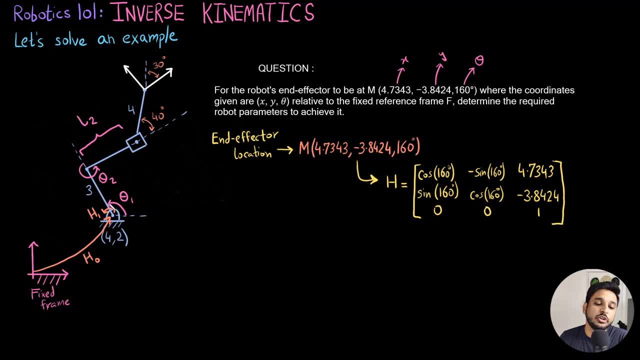 no displacement, only rotation. then there is a homogeneous transform that takes this h1 to this point, so i call this h2. now there is another homogeneous transform that takes this to this point, so i call that as h3. and finally, there is another homogeneous transform that takes this to this point, so i call this h4. 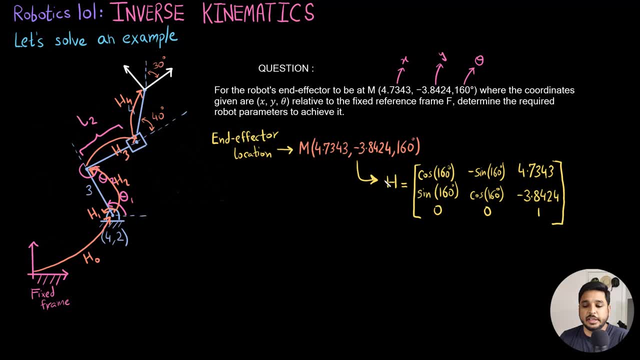 so you notice that in order to get this H, which is the final end-effectors position orientation, I go from H naught to H1 to H2, to H3 to H4, so I can write the forward kinematics in this manner. so forward kinematics is just the multiplication of H- naught. 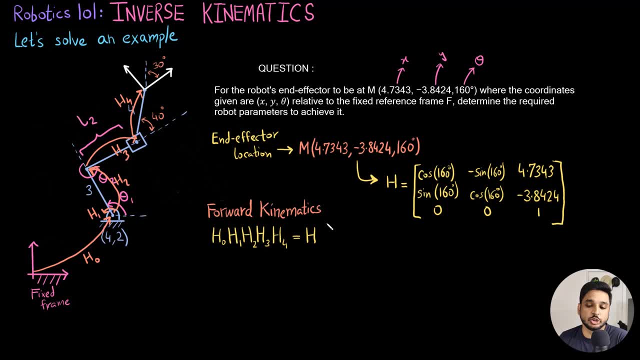 through H4, which is going to give me the H, which is this one. right here I have written down what each of the homogeneous transforms are. so this H naught is just a simple transition with no rotation. so I have put the rotation angle as zero. so I get an identity matrix right here: 1 0 0, 1. here the. 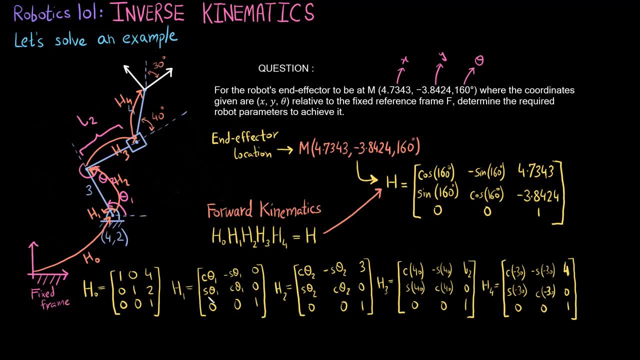 rotation angle is theta 1 and there is no displacement. in H2, there is a displacement of three units and X, 0 and Y, with the rotation angle of theta 2. in H3 there is a fixed rotation of 40 degrees, which is this one, and the displacement is L2, which is: 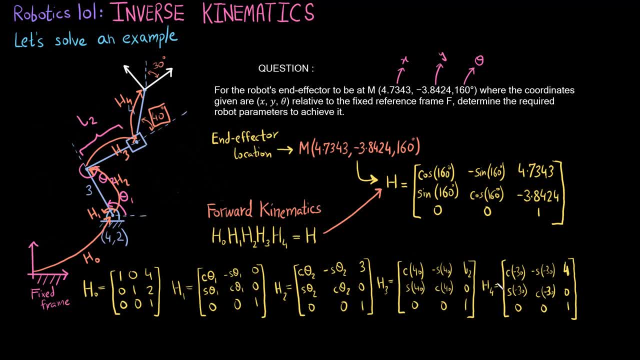 not constant, which can change, and the H4 has a fixed displacement and a fixed rotation. so what I notice right here is that what I need to find out is I need to find out the robot parameters, so I write. so what the robot parameters in this case are my two thetas, which are: 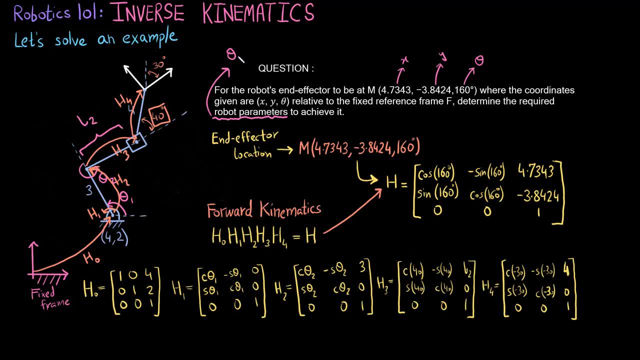 if I just write it down, which are theta 1, theta 2 and the third robot parameter is the length of this prismatic joint, this link, which is L2. so these are the three things that I need to find out: theta 1, theta 2 and L2, and if I have a 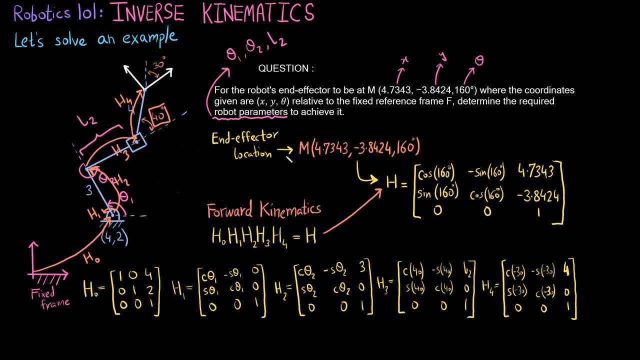 look at this homogeneous forward kinematics, I notice that these terms, theta 1, theta 2 and L2- appear in these three homogeneous transforms right: H1, H2. so, in order to simplify the problem, what we can do is we can take everything, which is everything. 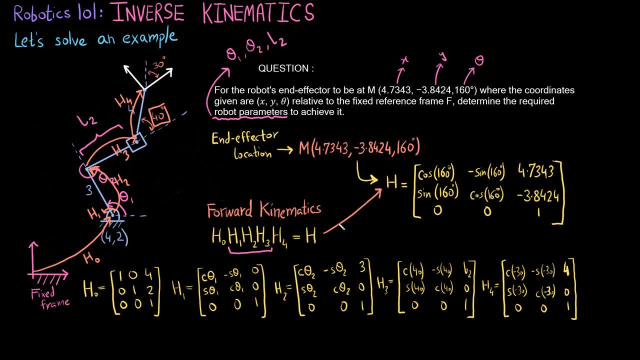 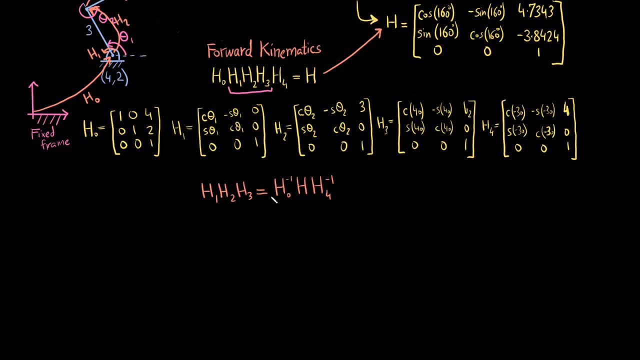 is on the left side to the right side. what i mean by this is that. so what we have done is we have taken h, naught and h4 to the right side. so i get this equation right here. what i've done is i have input this: h, naught, h and. 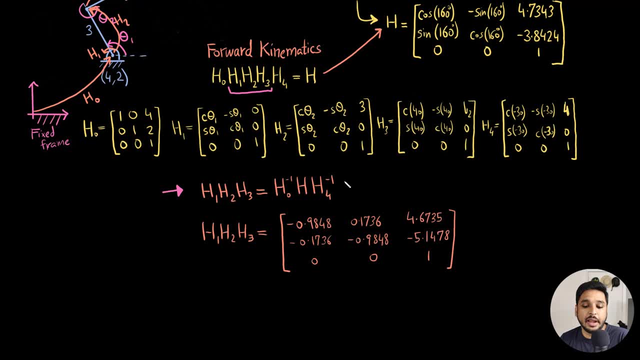 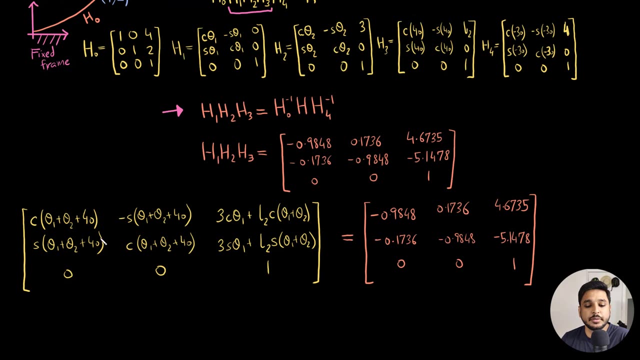 h4 inverse into metadata and i've gotten the solution as this. now i need to. so h1, h2 and h3. now if i multiply h1, h2 and h3, i got i get this matrix right here on the left, and this matrix is this one, and h1, h2 and h3 gives me this one. now i know that both of these matrices are. 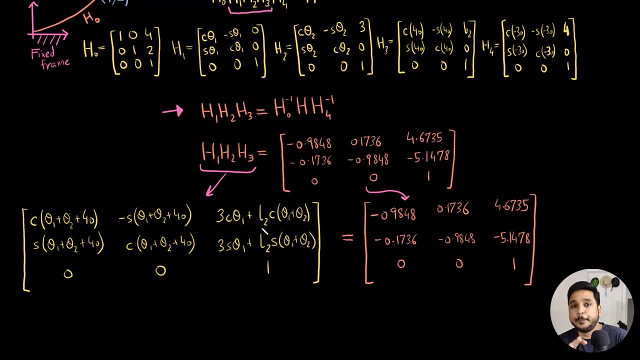 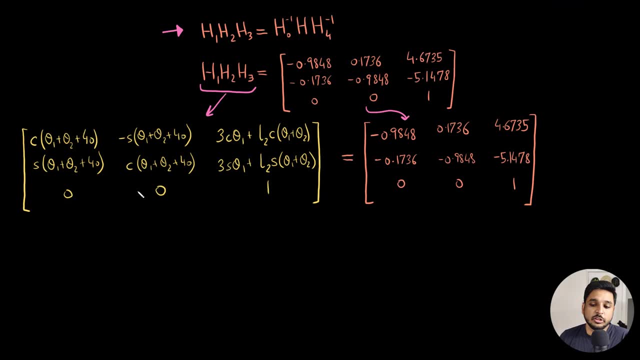 equal. so what i can do is i can compare the terms or across the two matrices. so if i start by comparing the terms, i can see that this has a sine and cosine. so what i will do is i will compare this sine and cosine with this term. so what i do right now is i compare the terms and i divide. 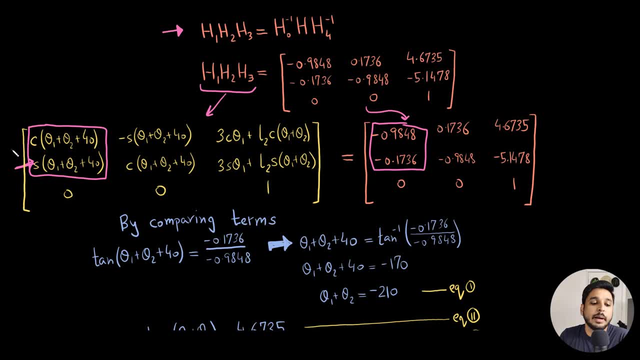 this term, the sine term, by the cosine term, and similarly, i divide this by this. so i end up with this equation: 10 of theta 1 plus theta 2 plus 40 equals to all of this, and if i just do a data manipulation, i take the 10 inverse. so i end up with this equation, which is: 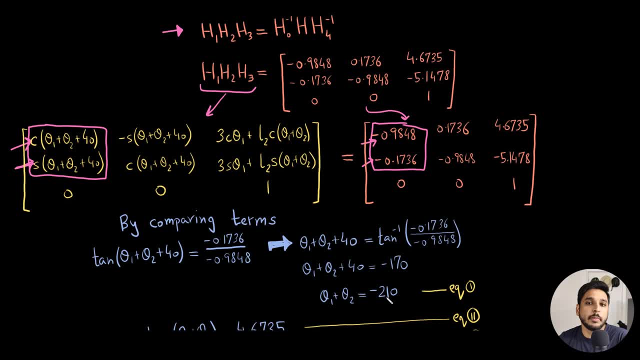 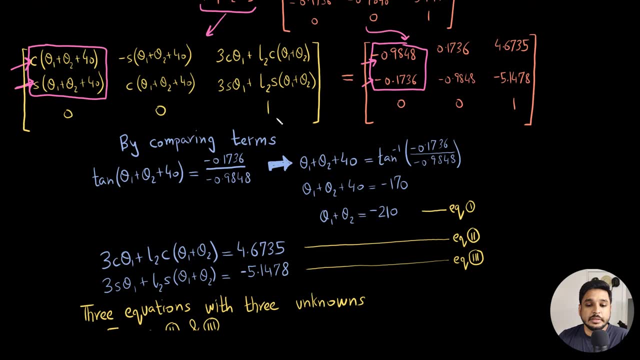 you equation 1: theta 1 plus theta 2 equals to minus 210. now, similarly, if i compare this equation right here with this, and if i compare this with this, i get equation 2 and equation 3. so now i have three equations with three unknowns. 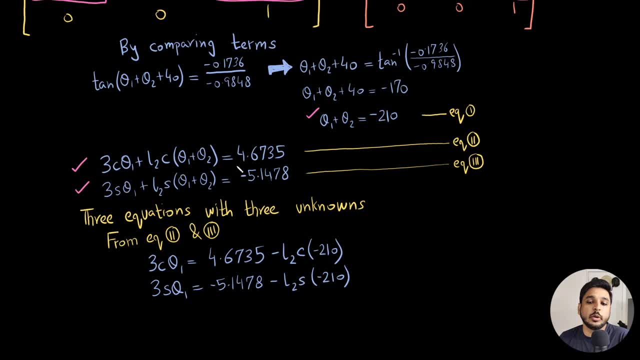 i have three equations with three unknowns and i know that what i need to find out is i need to out theta 1, theta 2 and a 2. so from this what i do is, from equation 2 and 3, i keep cos, theta and 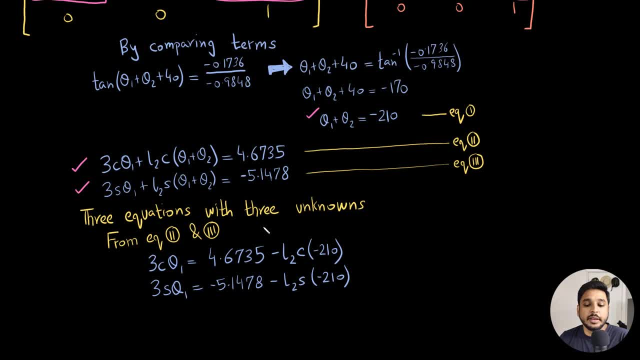 sine theta on one side and take everything else to the other side, and in doing so i realize that this is just theta 1 plus theta 2 and i already know the value of theta 1 plus theta 2 as 210 degrees. so i input this 210 degrees into this, so i get these two equations. 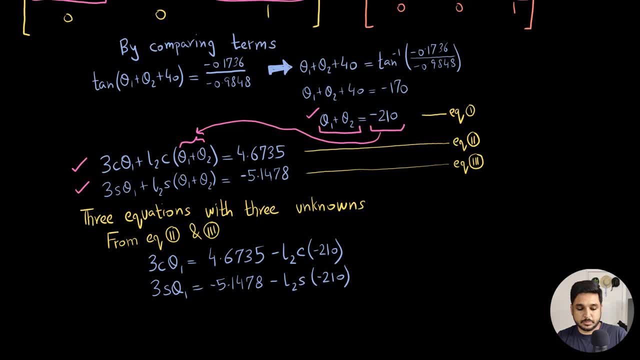 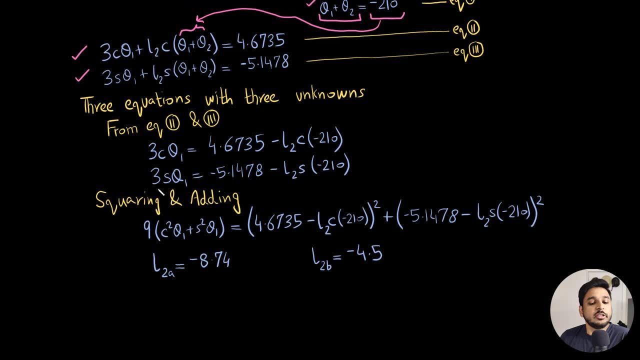 so now the way to go about it is: i take these two equations, i square them up and i add them up. i square them up and i add them up and, since i am squaring, i end up with an equation which has l squared terms, since there is a l squared term. so i get two different values of l2. 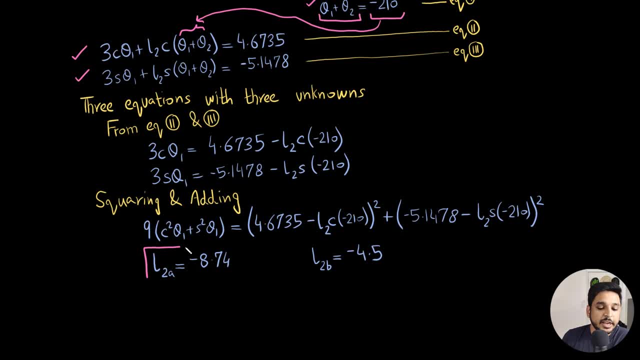 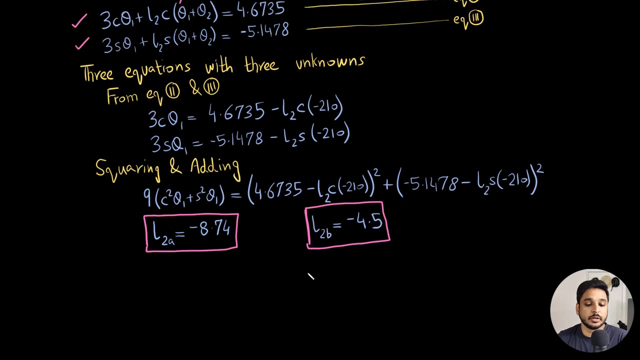 so the first value that i get is minus 8.74 and the second value that i get is minus 4.5. so what this means is it represents two different solutions of the link length l2. now the way to proceed is that i take this equation right here. 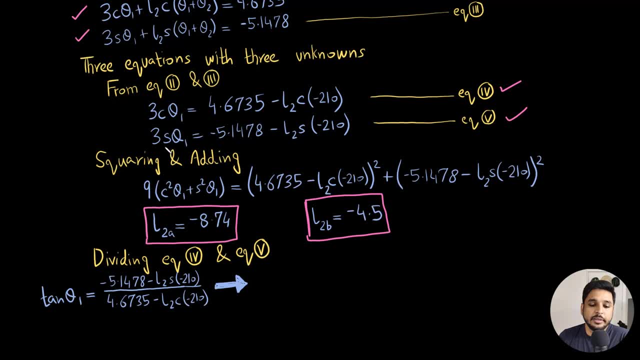 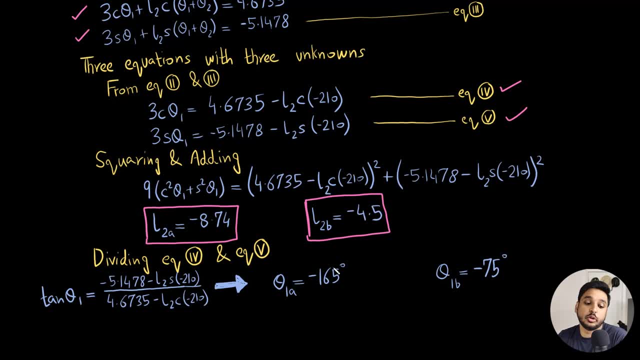 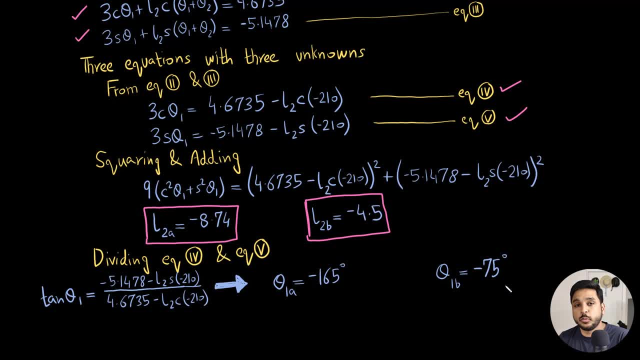 and then i input l2b into this and i get theta 1 b. so, similarly, i get two different values of theta one. so what this means is that this theta one- the first one, corresponds to this theta, uh, this a2 value and this one is working out messed up, because this one stands right. no, this one is. 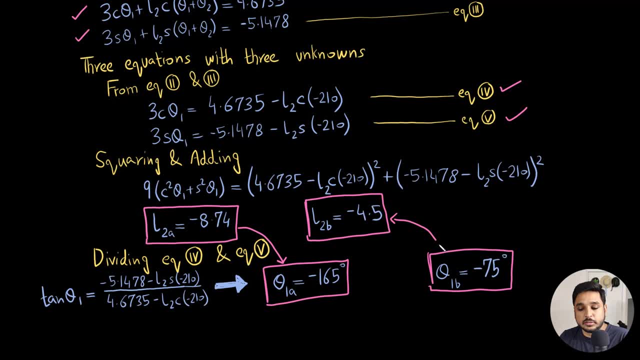 the first one being in. yeah, this one is always more correct. yes, this one is making do. theta 1b corresponds to this. so these two corresponds to each other. so a2a corresponds to theta 1a and a2b corresponds to theta 1b. now moving forward. now i already know a2a. 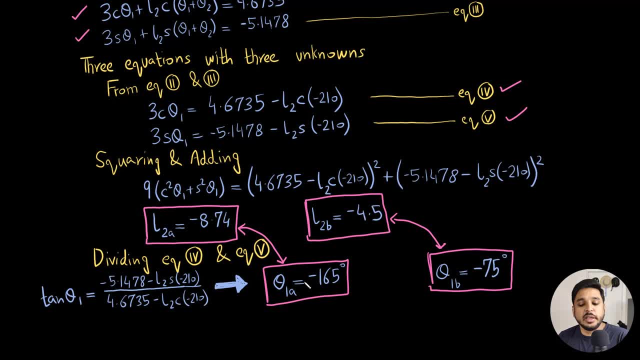 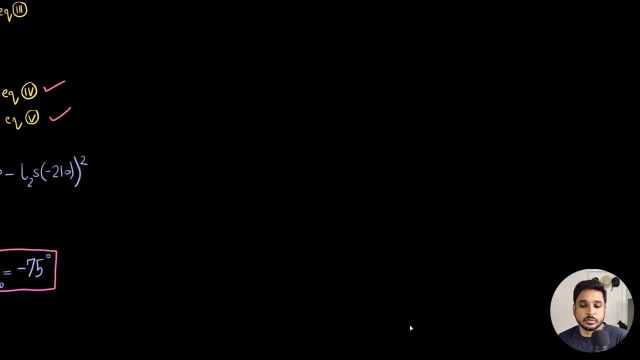 i know a2b, i know theta 1a, i know theta 2b, theta 1b, sorry. so i just need to find out one more variable, one more robot parameter, which is theta 2. so for that i use the very initial equation, which is this one, equation 1, which, if you require it, is theta. 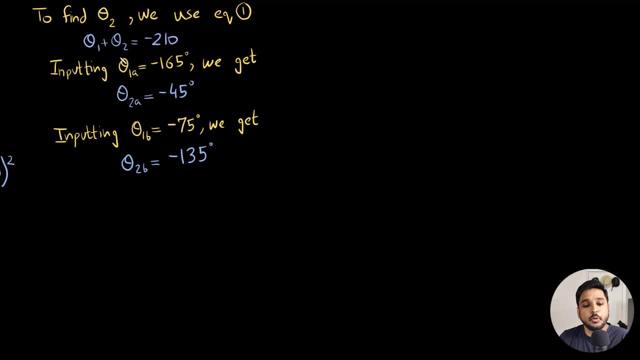 1 plus theta 2 equals to minus 210 degrees. so if i input theta 1a as 1, 6 minus 165, i get with. i get this solution for theta 2a, and if i input theta 1b as minus 75 degrees, i get this.